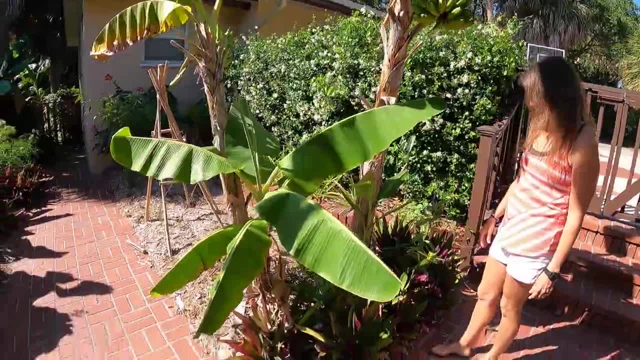 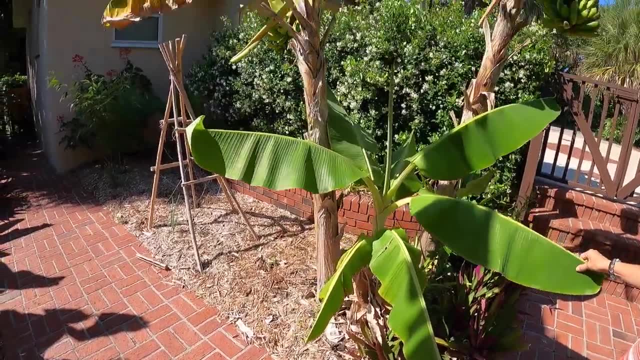 know it's not drawing a lot of energy off of the mother plant here, but here's another one we have. this is also a Mona Lisa and we actually allowed this pup to get big alongside of the the mother plant and you can see the rack on this one is is real poor compared to the other rack. 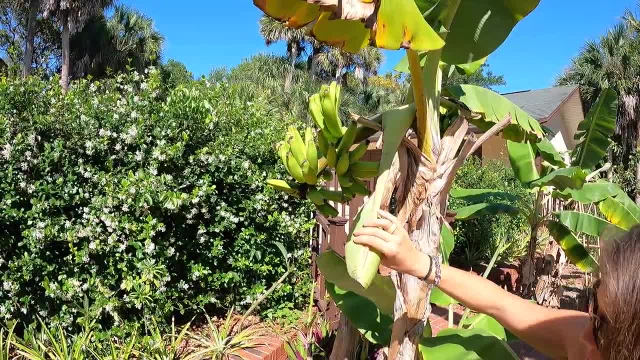 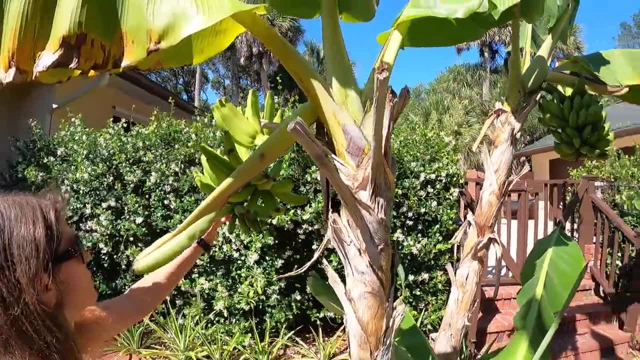 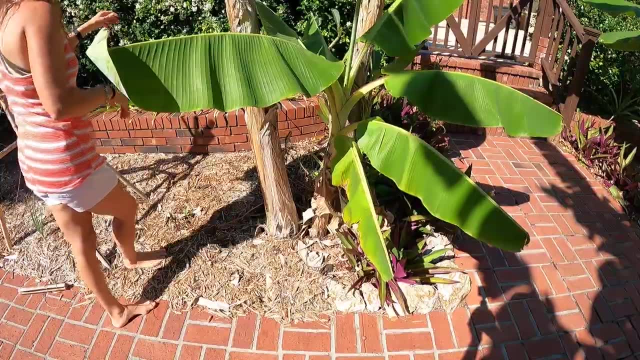 it's not even close. yeah, it's not different kind of banana, does the other one, in all honesty, is it? this is this one? this, this flower came out a lot sooner than this one did, so these are a little more developed than these are, but you know, this, this big sucker, this big pup right here, I, you know, I think, pulled. 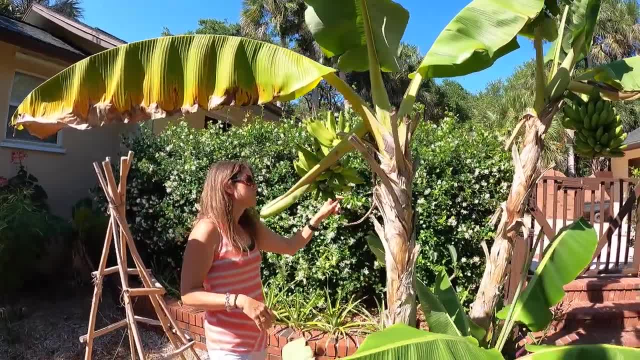 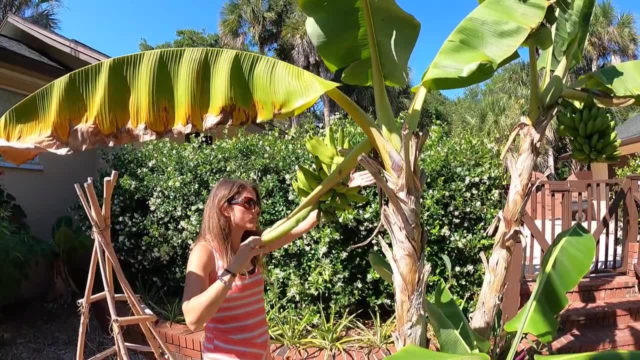 a lot of nutrients from the mother plant here and that's why we have kind of a poor rack and if there's another one, I never had these there's like: well welded, they're welded together. yeah, they are fused, and that. that one never had that when we 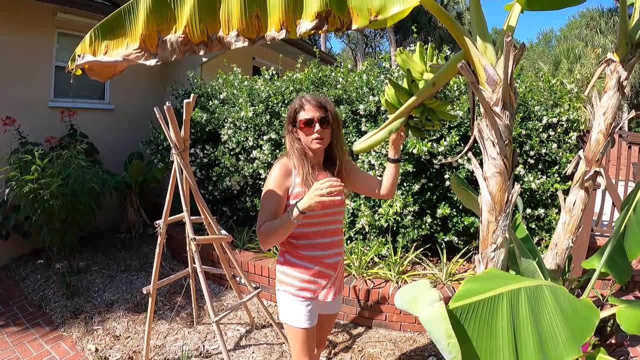 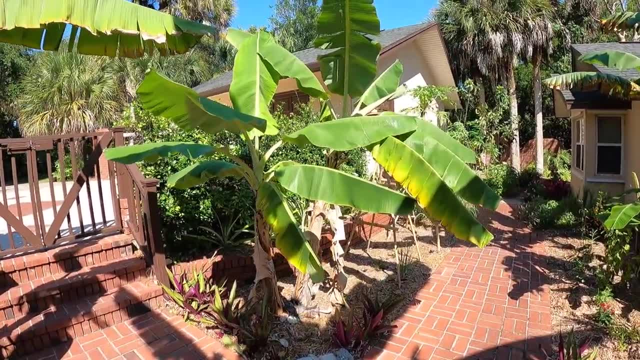 saw this come. we thought it was a different kind of banana because it looked so different. so we have another rat. we have another kind of banana over here. this one we just called the ralph banana because we got it from our friend and neighbor ralph. but we did the same thing here. we didn't. 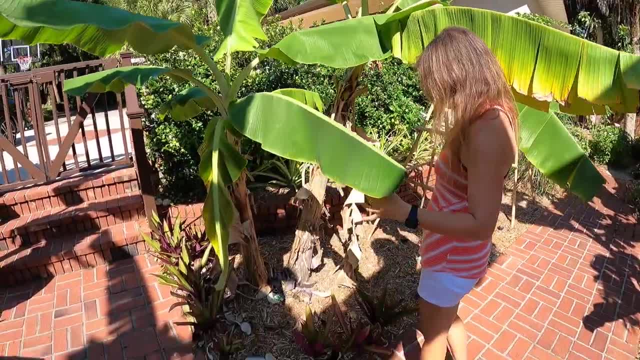 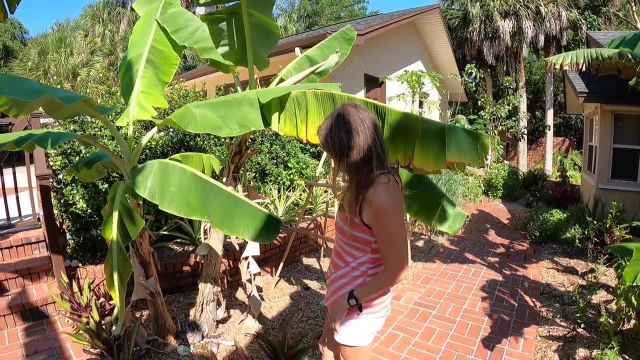 separate this big pup from the mother plant because, um, we we really wanted to have one of them live. um, i didn't. honestly, we didn't care about the rack of bananas that came off this the first time, because we wanted the variety of banana, so it didn't matter if we got a good rack. 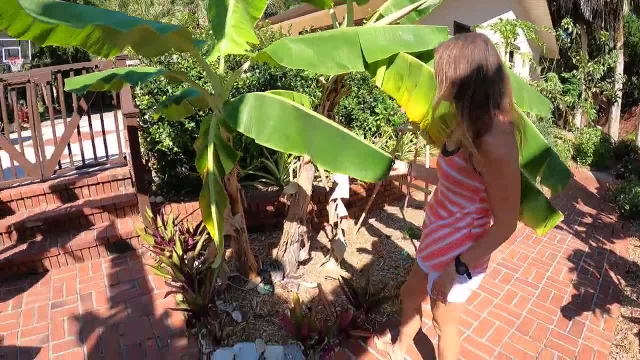 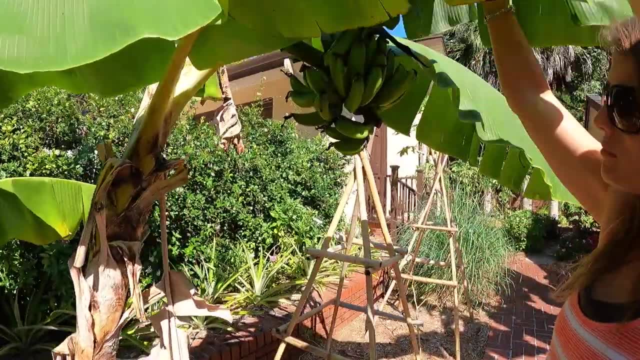 or not, but because we transplanted it pretty big, we did well. the and the two of them were already together, but because we didn't separate them again, can you lift that up so they can see? this rack right here, you can see, just is not as nice, there's not as many bananas and they're not. 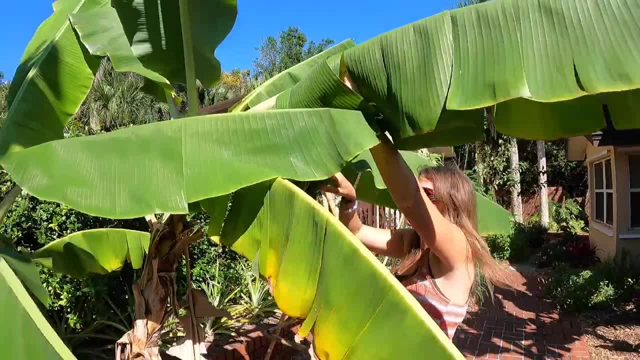 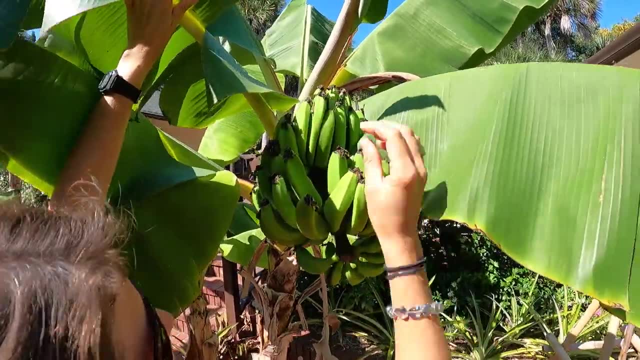 as well welded together. yeah, they're like. if you look, come over on this side, you can see how, like the bananas, yeah, they're just not round. i mean let's get started, get a close look at this and then let's go over and show them this rack again over here. i mean. 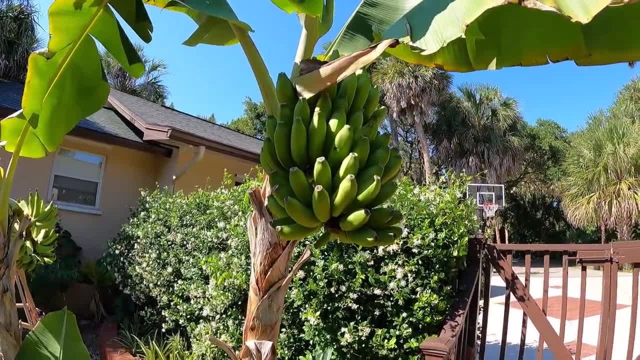 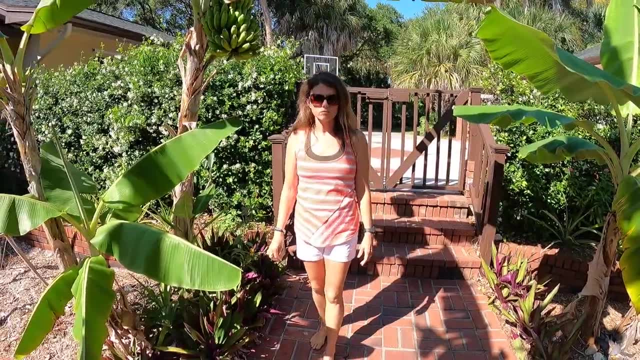 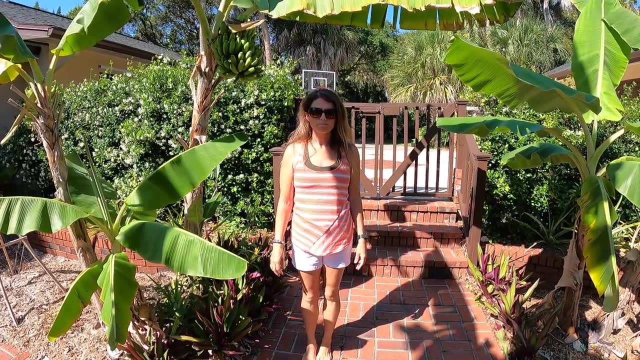 it's just the two don't even compare, and so really, that's the first. that's the first reason why we think you should um thin out or separate your um banana, your banana pups, and we actually um just went for a ride around our community and um got some footage of some big stands of banana. 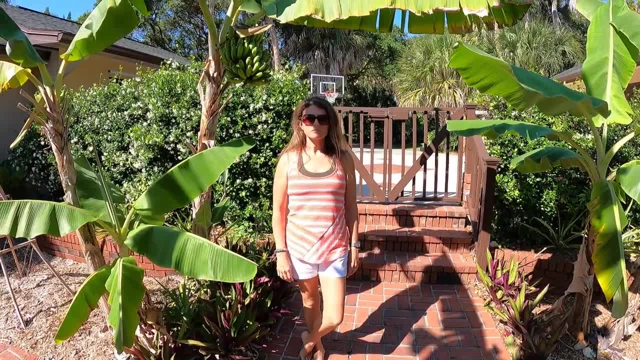 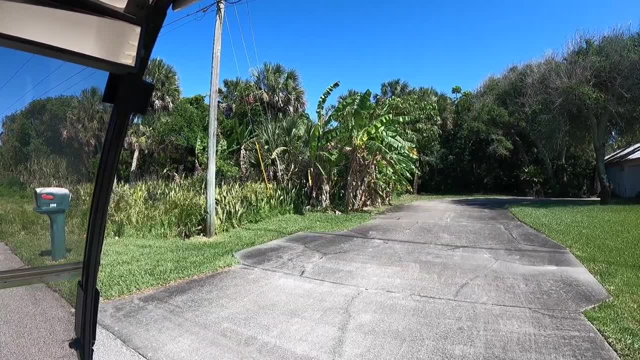 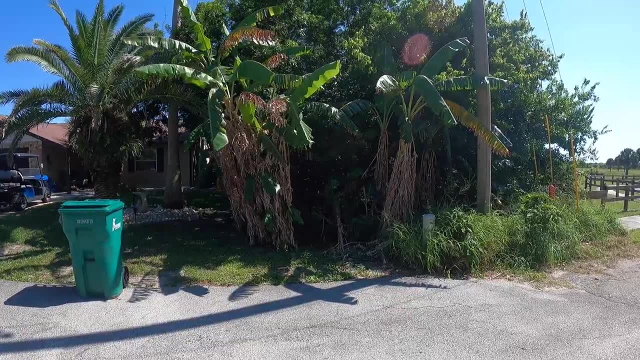 plants. um, there's lots of banana plants in these stands with no bananas on them, right, and so we'll show you guys that footage right here. here's an example of a lot of banana plants and not a lot of bananas. here's another example of a lot of banana plants but no bananas. 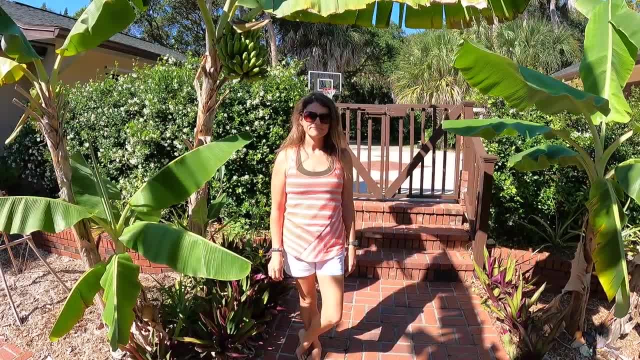 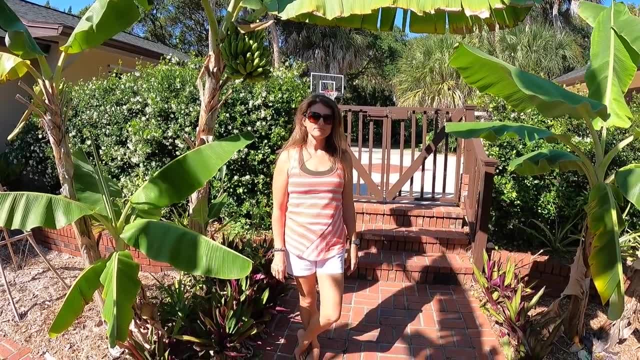 and so you, you could see um both of those stands that we just, we just showed. i mean, there was probably what? 20 or 30 plants in the first stand, maybe less in the second stand, but there wasn't one rack of bananas on on the next stand, so there's a lot of unplanned houseplants in that stand. 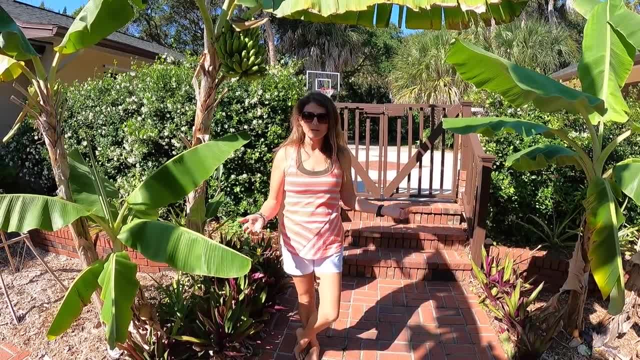 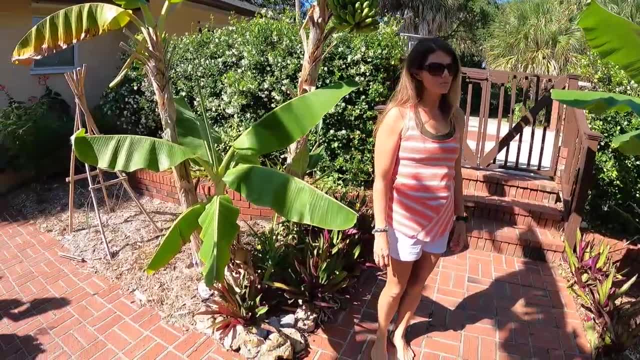 and that might be what they're going for. yeah, they might just be going for bananas, you know, and they just like the way, the banana plant. so that's, that's right. yeah, so that's the first reason why we want to encourage you to, you know, separate these pups from the, the mother plant. now, 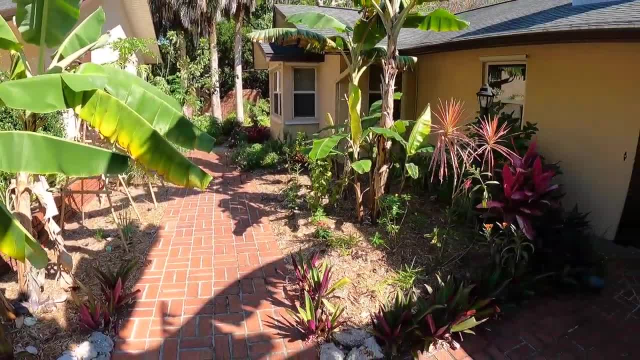 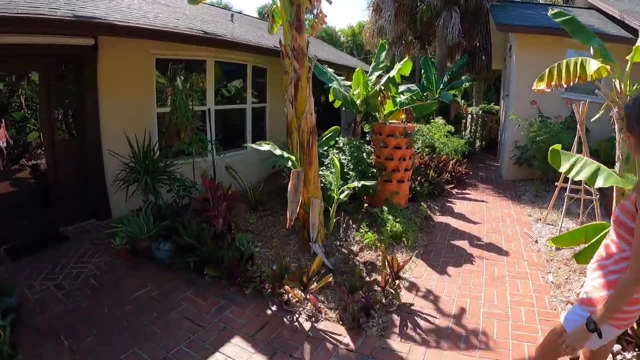 you know also, we have a second reason here and if you know you can tell almost right off the bat: these, some of these varieties of bananas we have, are massive and i mean we just don't have room in our garden for all of them to grow up. i mean we, we just don't have the room. so that would be a 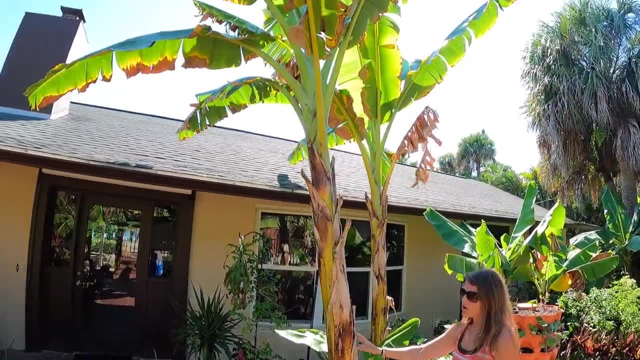 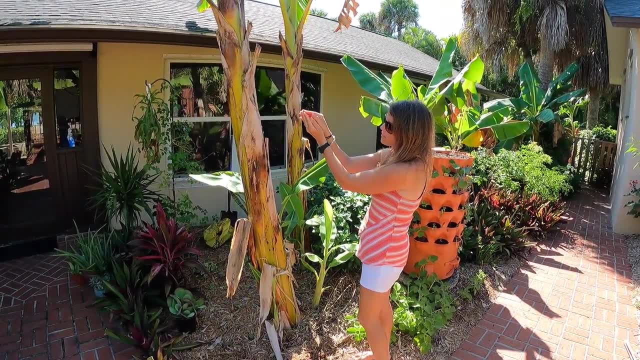 second reason why you might want to separate your pups from the mother plant. these are all real special varieties, though. um, this one is called the praying hands and the bananas, um, kind of face each other, so this will be a really exciting one. i'm so excited for this one, so i want to make sure that 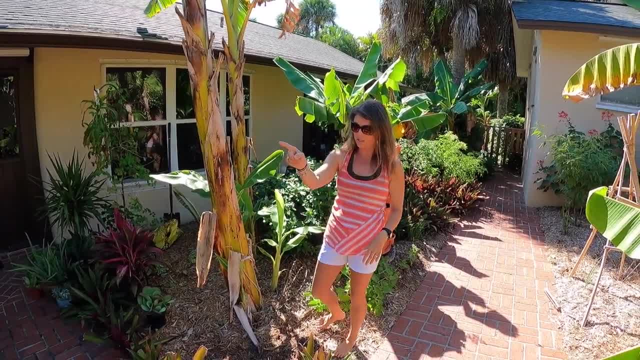 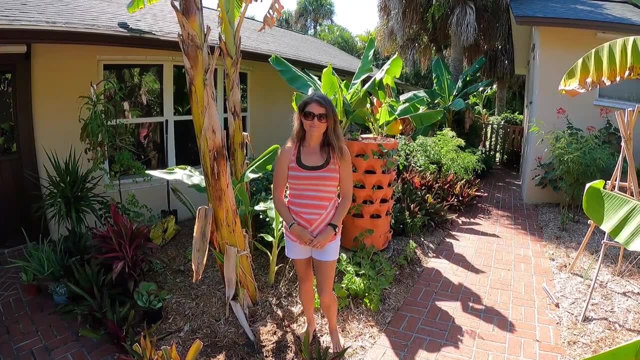 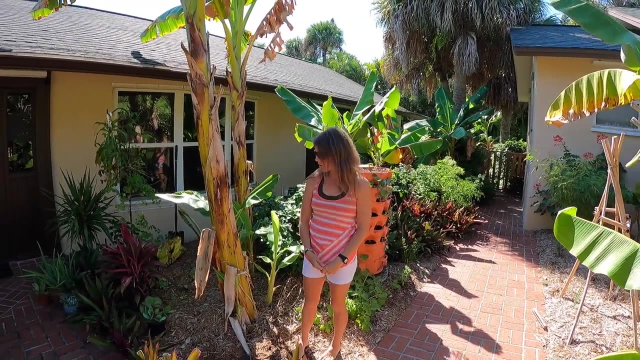 the bananas that come off of this one. so that's that one is a special one too, right? so that's banana. so that's the third reason why we want to separate them is to get more banana plants, right? so you, these are, these are all special varieties that we've collected. so so, um, so there's a couple reasons. 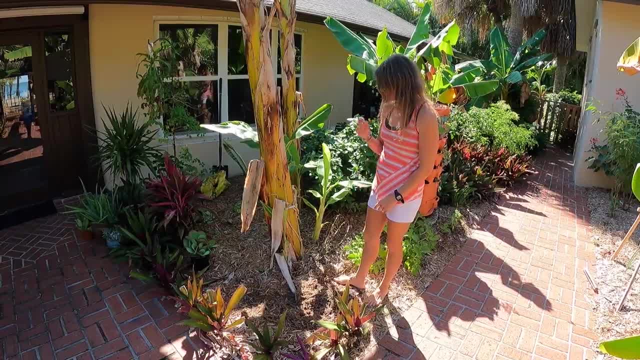 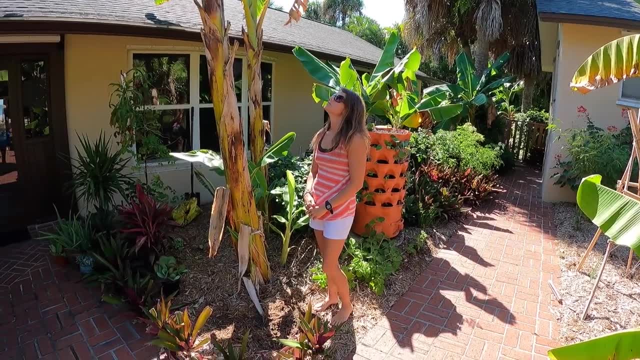 why you want to. you know, separate them, remove them. now you know. so now let's talk about when. well, you know, if you just don't care, this is going to sound crazy to some people who don't have a lot of bananas, but you know, we have so many pups we're probably just going to hack some of these off and 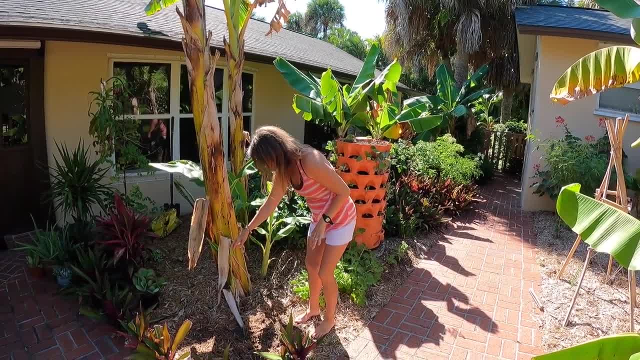 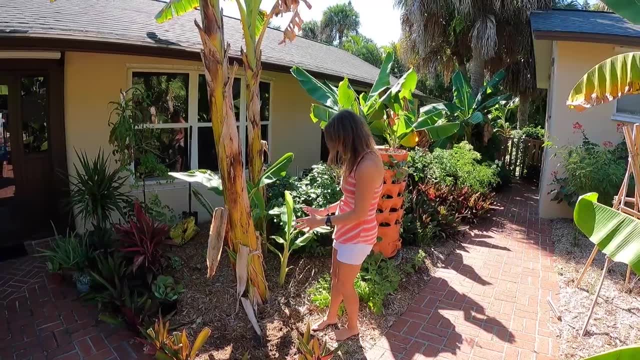 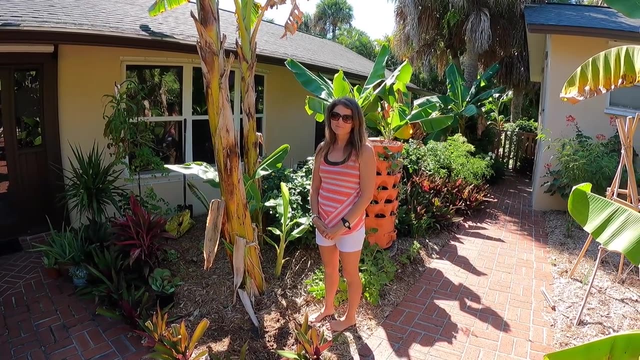 throw them away. right, we have, because we're this one we're going to just roll the dice with, because we really want these bananas to have all they can have when they, when it flowers, and we we're trying to have different varieties of bananas around our property and we're trying to keep them all separated, so we 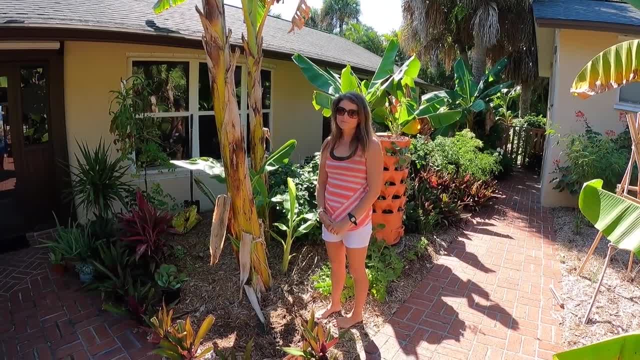 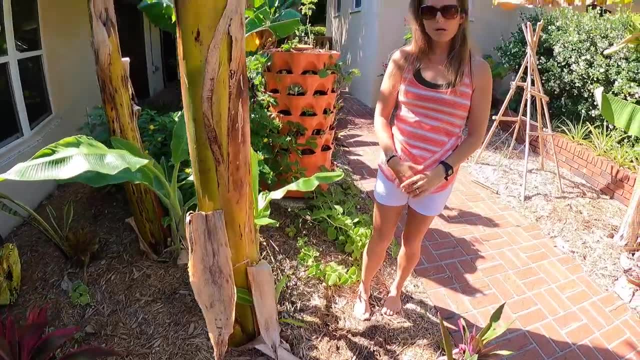 can't plant every one of these, you know, it just doesn't make sense. so, as crazy as it sounds, some of these beautiful specimens here are just going to probably own it, i don't know- in the final space this round. so, anyways, if you want to move one of them, you know, obviously you if you have a choice. 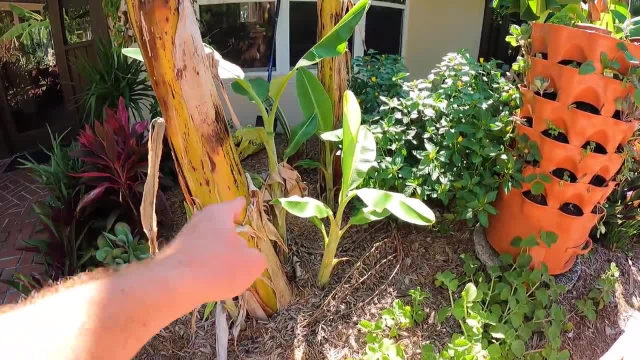 you want to pick one that's probablyasteempольше, probably just going to pick one of the other two around. you know, obviously you, if you have a choice, you want to pick one that's probably just going to, that's probably developed some, you know some good roots like this one back here. i mean this one. we 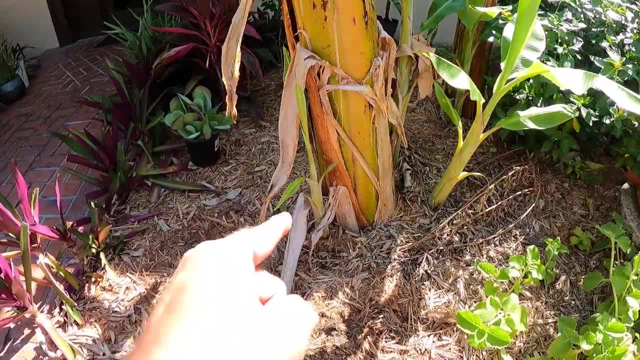 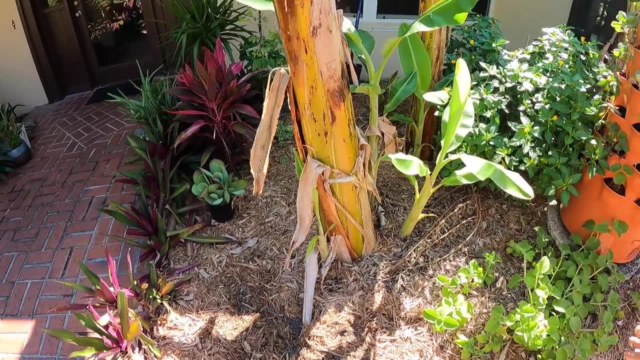 might be able to move. but you know, if you're moving this just for the sake of the health of the mother plant, i would just say whack it off and whack it down and get rid of it, right, but i mean. but if you want to move it to save it, you know you might want to let it grow up a little bit. when they get this big, they're still not drawing a lot of energy from the mother plant. so i mean also, we found, even when you do sacrifice these, they pop back up. yeah, yeah, and that's another thing. yeah, we're gonna- we're probably gonna- get rid of all of these pups on these and they'll. 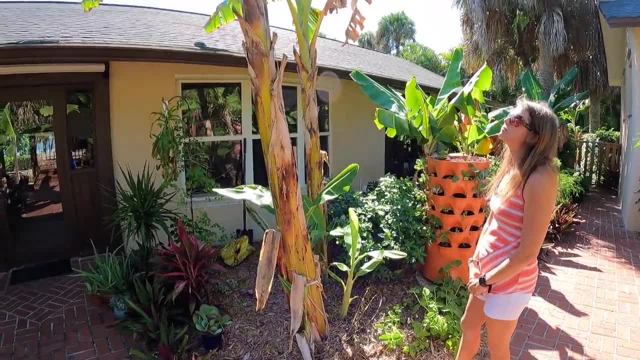 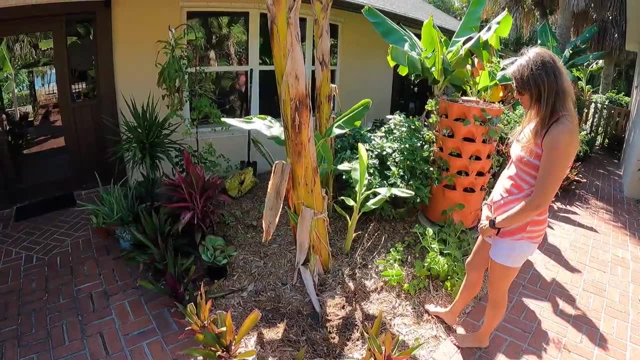 this mother plant. even if it doesn't pop one up before it shoots up out of flower, it will have a pup. before we hack the whole thing down to the ground, um, we'll probably chop and drop all of these, you know, once the bananas are done forming so well, let's go ahead and show them how to remove. 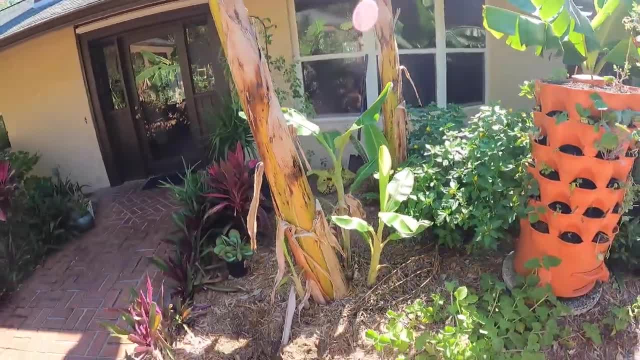 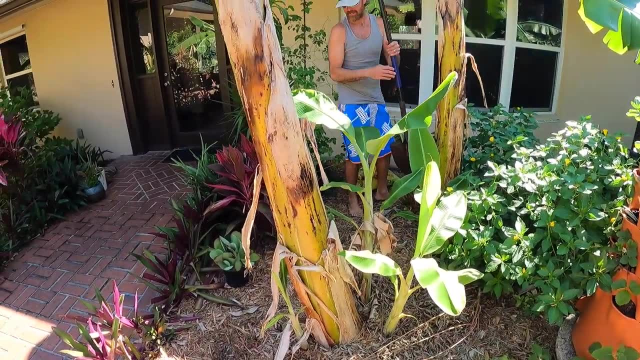 one of these. this is: um, you want to do it? yeah, i'll hand that over to you, and so what we do, i'm going to go ahead and remove this one right here, i think, because it's a good side and it's pretty easy, it's? it seems a little scary. it's your prize banana plant to do this, but 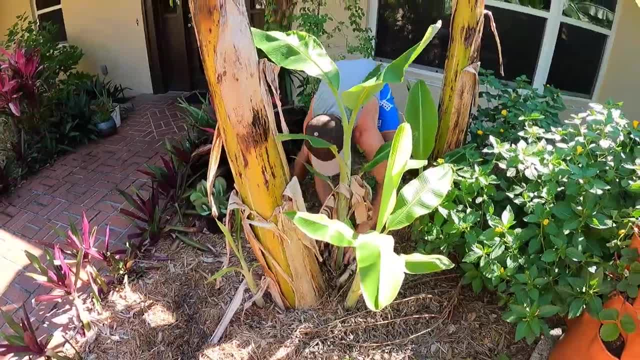 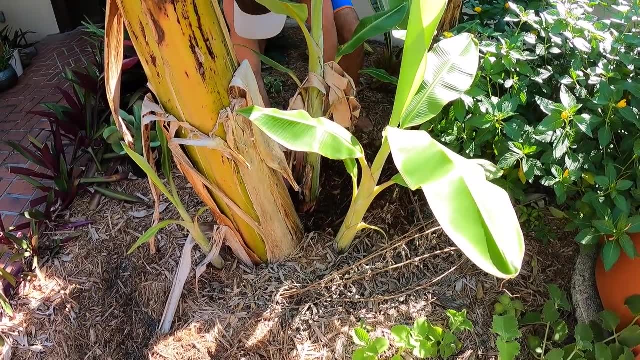 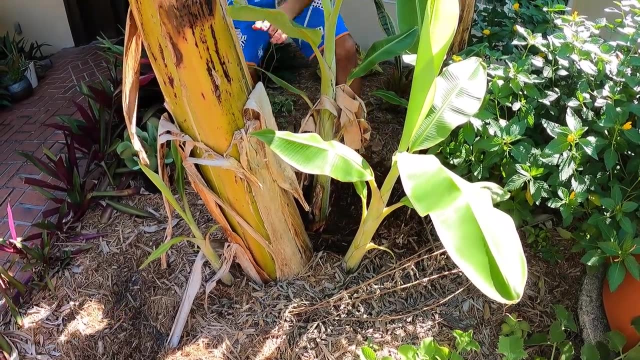 i promise it won't hurt the plant. so i'm going to kind of move all this mulch back here. and i want to move the mulch back a ways because i don't want mulch to fall down into the hole we're about to make. we want to kind of keep just dirt in there, so and then we'll kind of just wedge. 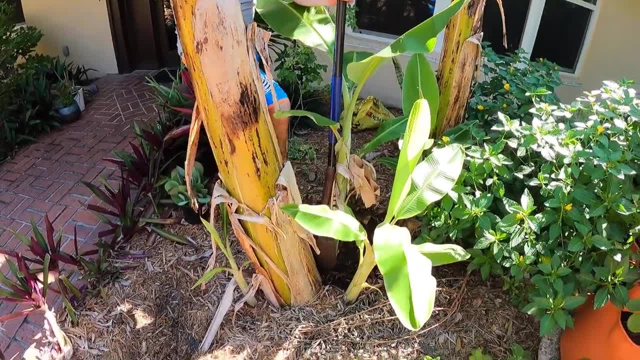 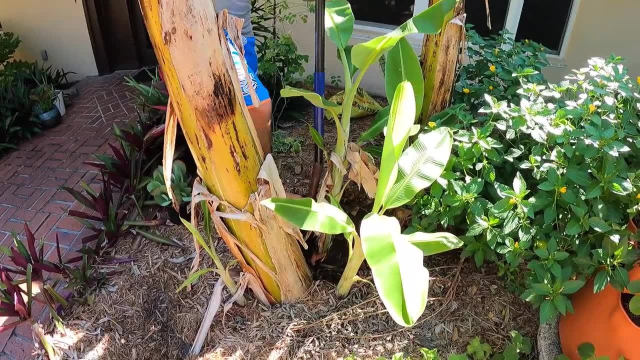 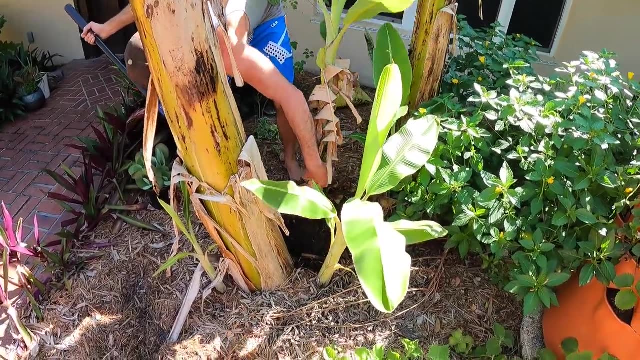 the shovel in between the mother plant and the plant, and we're going to go ahead and do this, just kind of pop and just kind of shear it off, and you don't want the mulch going down there because it'll create like air pockets and can make your roots rot. all right, so i didn't get a lot of, you didn't get a lot of uh. 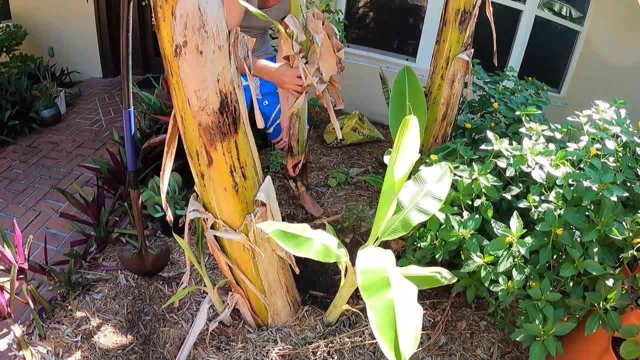 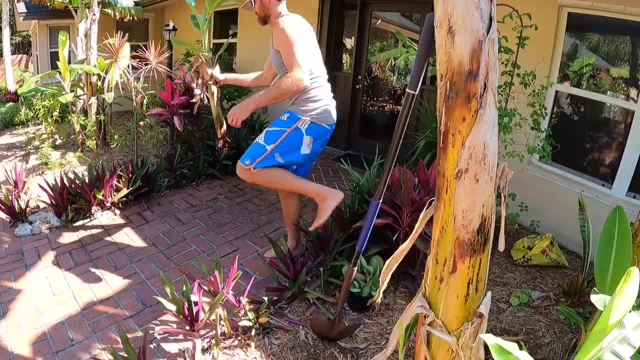 roots off of this one. but, believe it or not, it's really okay. we can probably still plant this and be okay. and then what i'll do is, uh, let me just set this down over here. what i'll do is i'll just come back in this, this one, and i'll just set this down over here, and i'll just set this down over here. 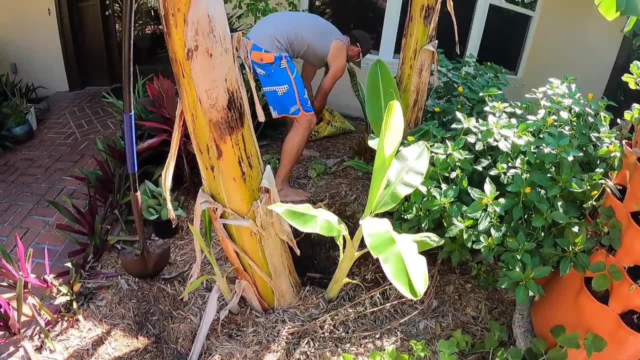 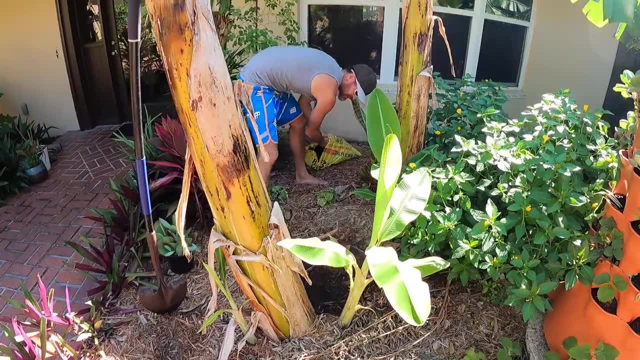 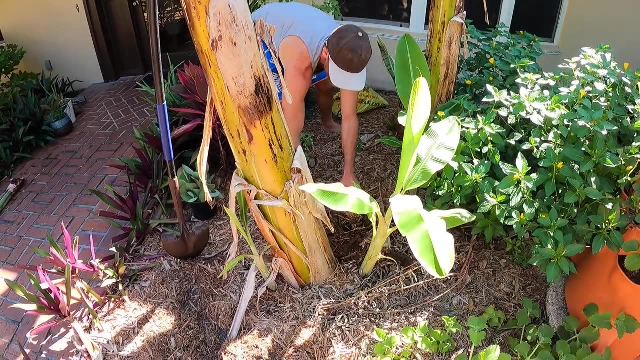 hole that we just made here. I usually pack it with just some, some compost or cow manure, you know, I don't know, just even dirt, just to give the the wound a little extra nutrients here, and then we'll just put the mulch back. so and 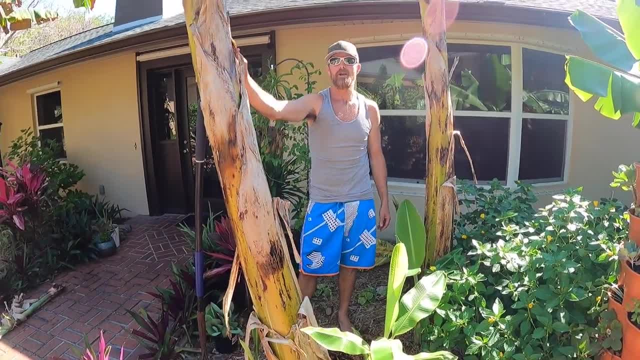 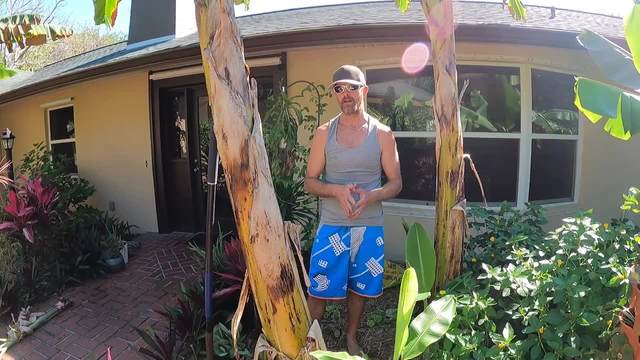 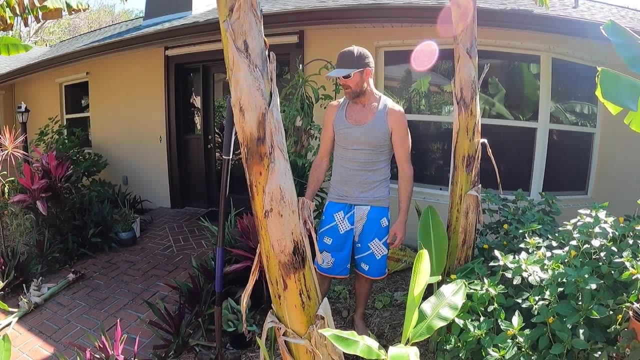 we'll probably go around and do like I said: we, we like these, right, you want to move these somewhere else? yeah, so we'll probably take two or three of these nicer pups and move them to a different area, and then this little one, we'll just get rid of it and or try to let it go. and so then you know, because we have all 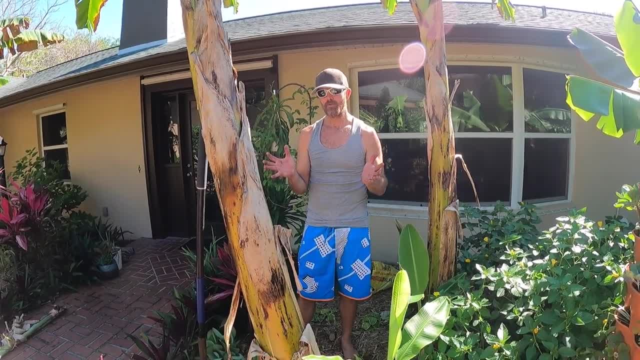 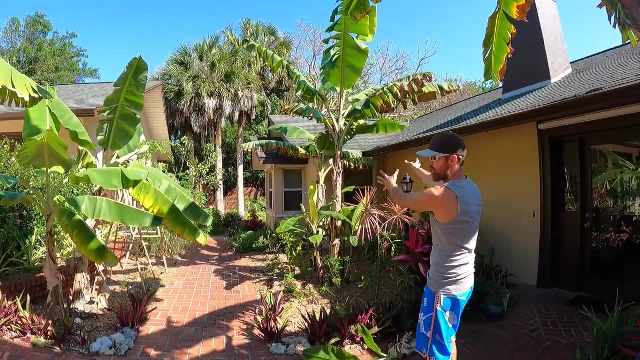 these different varieties. you know you got to keep them obviously labeled, but you got to keep them separated too. you can see how we have them. you know we don't have two different varieties right next to each other. these are all one variety. these are all another variety. these are all another variety because 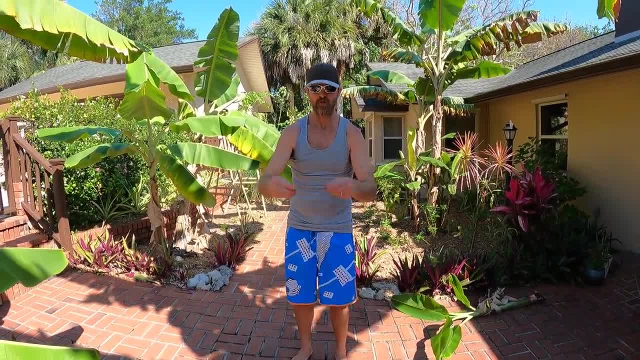 you know, if you plant them right next to each other, they're not going to grow and they're not going to grow. and then you get a bunch of pups that are spread out very close to each other and pups shoot up, you know, between them it's. 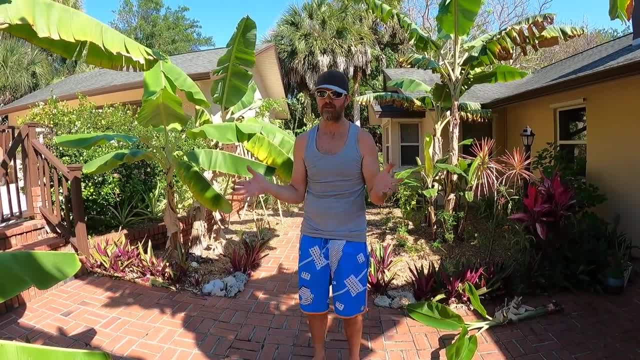 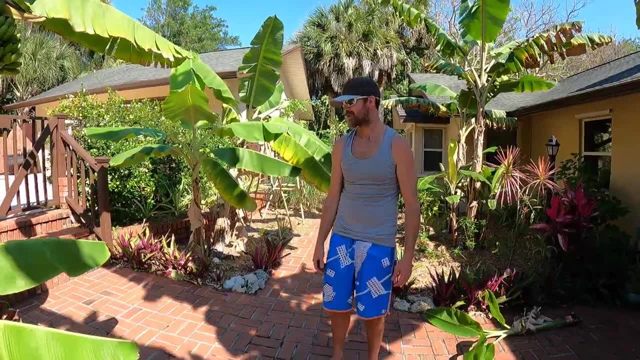 going to be hard. the pups- some- usually the pups- shoot up right off the base of the plant, but sometimes it's a foot away, you know, and if you have two different varieties right next to each other, you might lose track of which variety it is. but maybe you could come up with a new kind of banana. but yeah, alright, so we're. 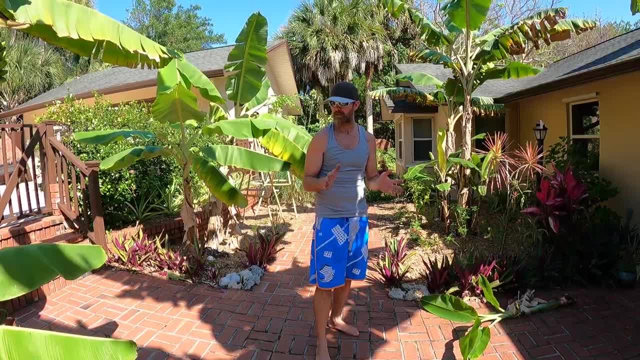 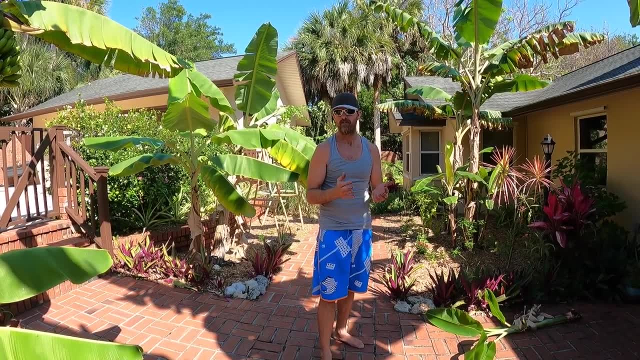 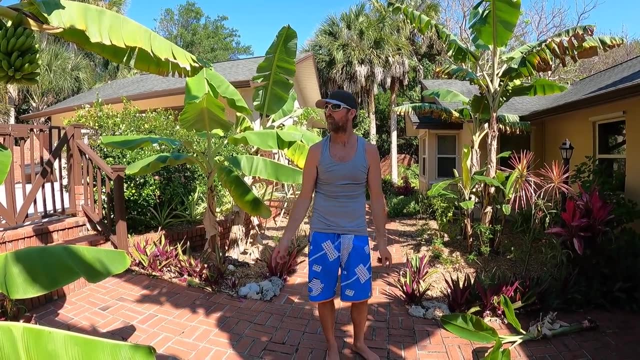 gonna go plant this somewhere that we just wanted to do a quick video about. again, we we've seen a lot of, you know, big stands of banana plants around here that haven't been separated. you know big, bushy stands of banana plants with no bananas on any of them, and we're growing them for the bananas.